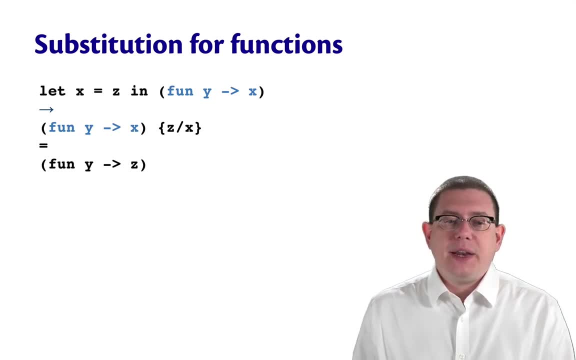 works with these functions. Suppose I have a binding let. x equals z in the first of those functions, the blue one: fun y, arrow x. Well, according to the semantics of let, that's going to step to fun y, arrow x, the body expression with a. 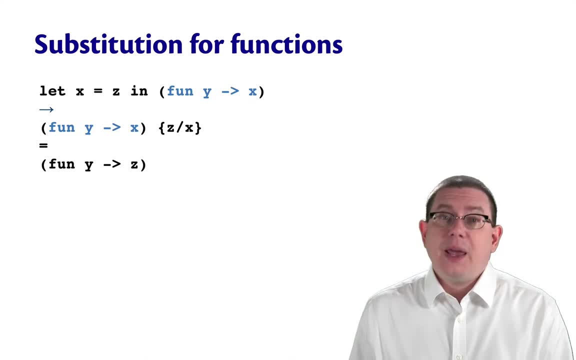 z substituted for x And, according to the definition of substitution for anonymous functions we just gave, since y and x are not the same variable name, we should go ahead and do the substitution of z for x inside of the function body. That would give me the function fun y arrow z That's going to ignore its. 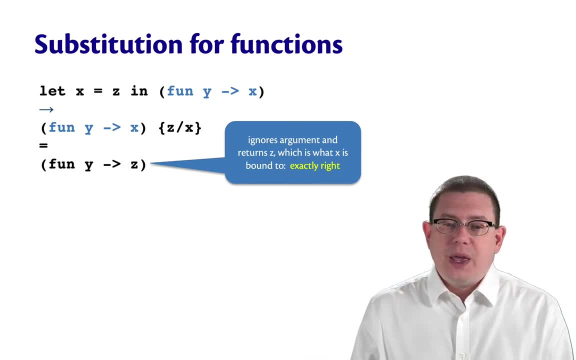 argument, which is what we wanted these two little functions to do, and it's going to return z. Well, z is what x is bound to, So this is exactly the right thing. This is what we wanted to have happen. In the end, the right value is being returned. 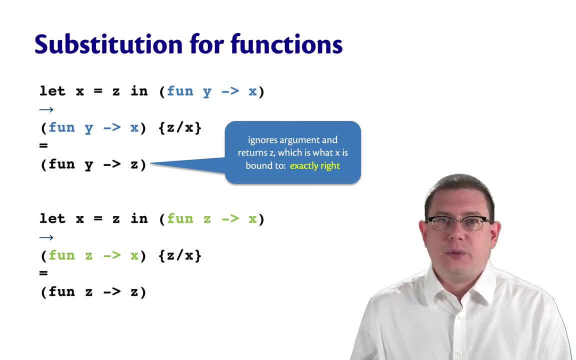 Now what about the other function, fun z arrow x, which I put in orange? Well, if you work through the definition of substitution here, we're going to get to substituting z for x inside of that function, But since z is the argument, 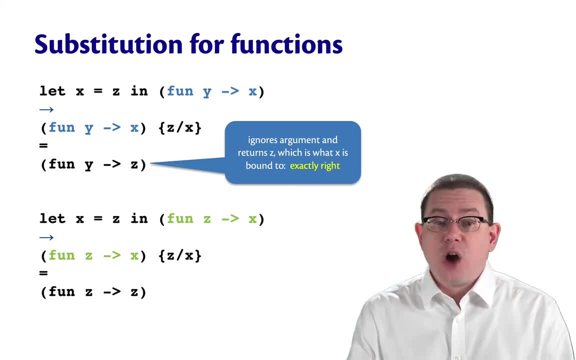 already being bound by that function. we're going to stop and not recurse inside of it. But look what just happened. We got the identity function at this point. This function does not ignore its argument. It returns whatever's passed to it. So these two functions are not the same function. They will not behave the same. 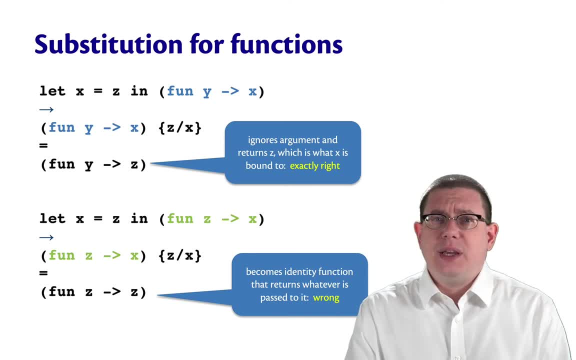 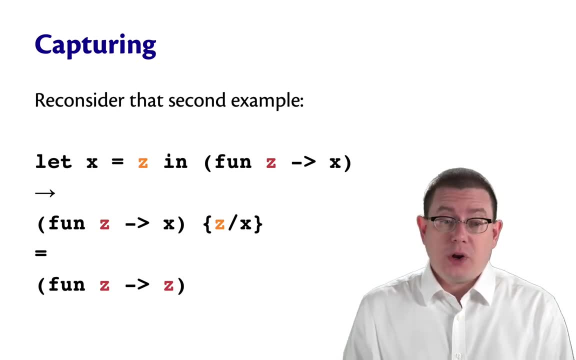 way in all contexts. There's something broken here with our definition of substitution, So let's take a closer look at that second example. I've color coded the variable name here, z, to indicate the difference between where it's being bound. The orange z was 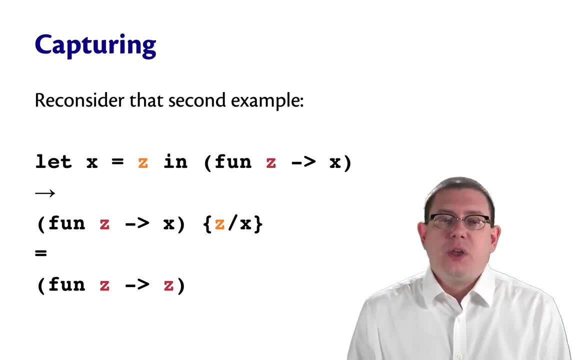 bound somewhere outside of this scope. We're not showing it here. The red z is being bound by the function. When we do the substitution, we're letting the orange z get clobbered by the red z. The technical term here is captured. 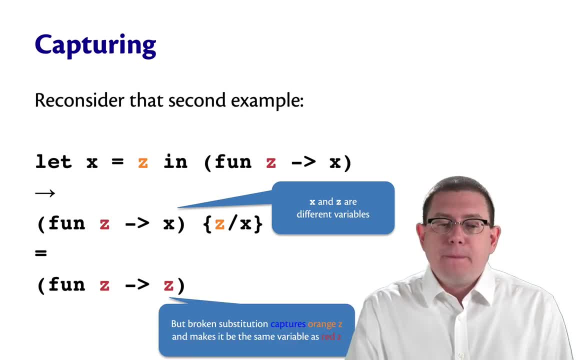 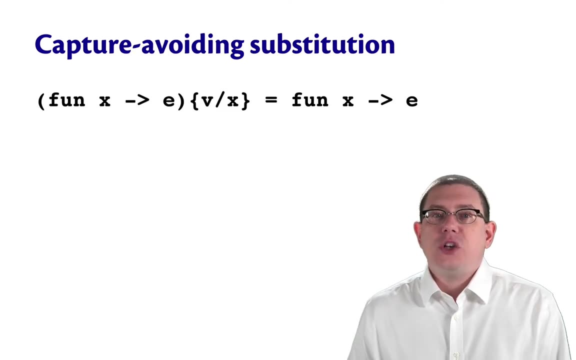 x and z are actually different variables, but the broken definition of substitution captures the orange z and makes it be the same variable as the red z. It breaks the way we expect scope to work. So we need an improved definition of substitution that avoids doing this kind of variable capture. 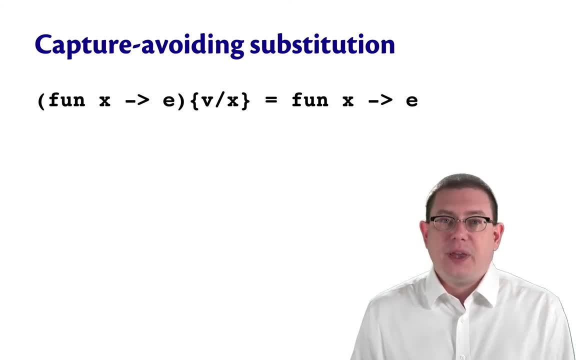 It's called capture-avoiding substitution. Here's the definition of it. When we do a substitution inside of a function- fun x, arrow e of v for x- then, as we've seen already, we go ahead and stop substituting at a binding of the same variable name. 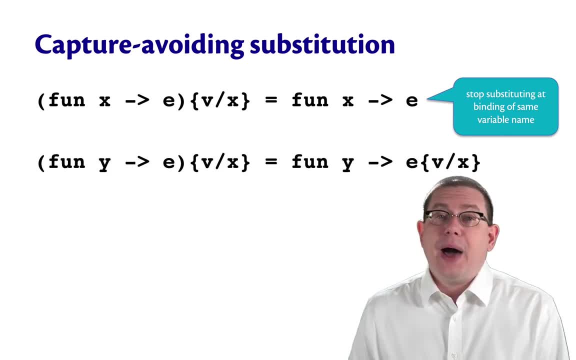 That's the same as we've always seen. But when we try to substitute inside of an anonymous function that binds a different variable name, we will go ahead and recurse, but only in certain cases. We'll continue substituting inside a binding of a different variable name. 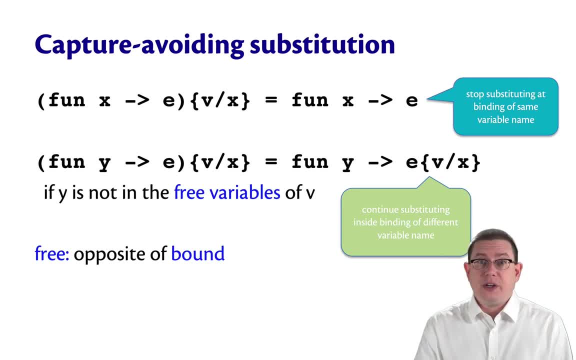 if- and this is kind of like a precondition- if y is not in the free variables of v, Okay, so what's a free variable? Free is the opposite of bound. You know what a bound variable is? It's one that's showing up as being bound by a let expression. 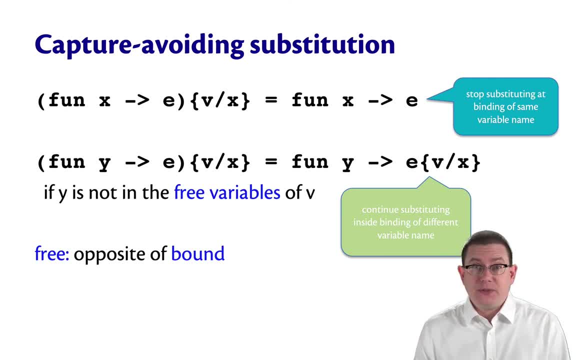 or bound by a pattern match or bound by an anonymous function. So a variable is free if it's showing up and it's not been put into scope by any of those. So we don't recurse inside the body if v is not in the free variables of v. 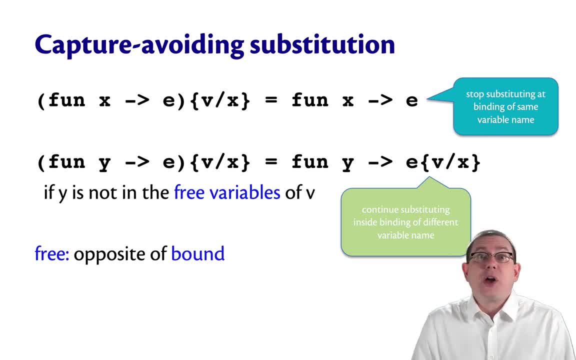 If v has a free occurrence of y in it, because that would cause that y to be captured just as it was earlier with the variable z. That makes this a partial semantics, in the sense of a partial function. There are some cases where we simply can't use this definition of substitution. 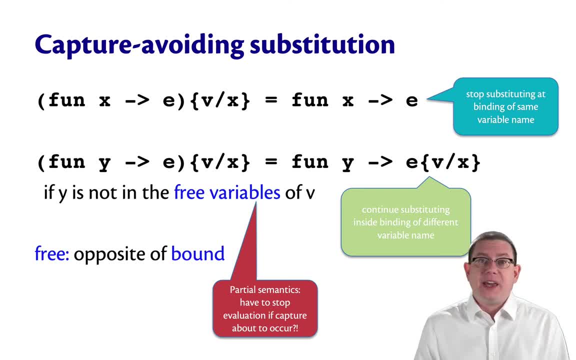 because we have free variables inside of v that would get captured, and we're sort of stuck at that point in doing the evaluation. So do we have to stop evaluating? Well, the answer is no. Instead, if we're ever about to capture a variable,